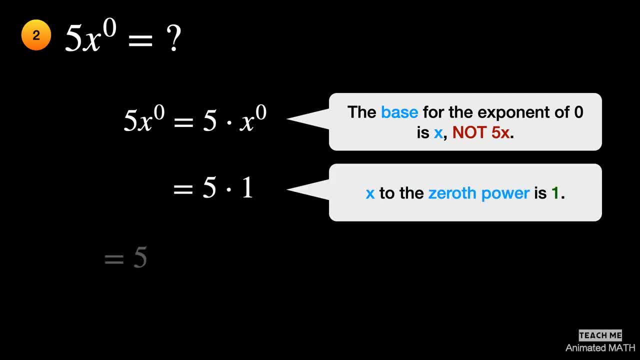 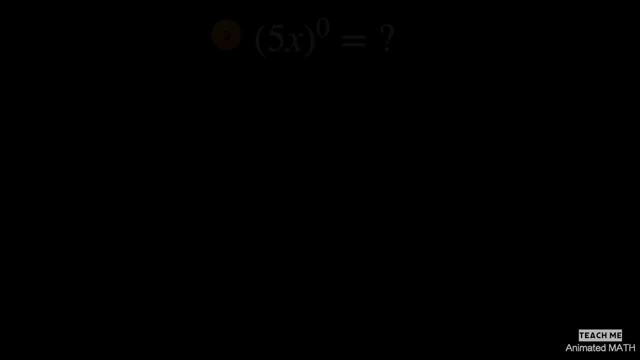 The bear is an exponent from zero to the zeroth power. Therefore, X equals the length of a zero. So why was the value of zero in theわ's argument a zero's exponent? Here we are. How about a愀 expression? 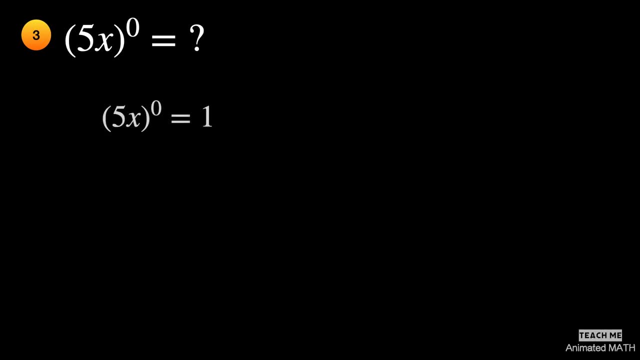 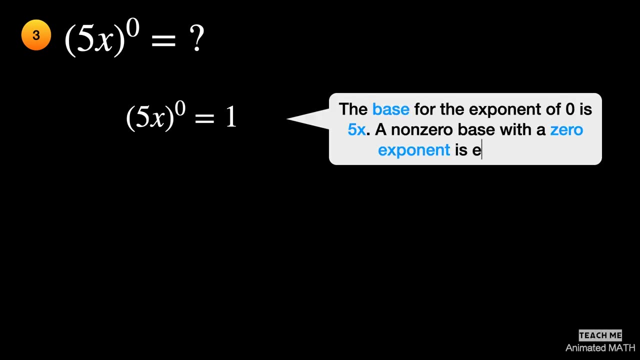 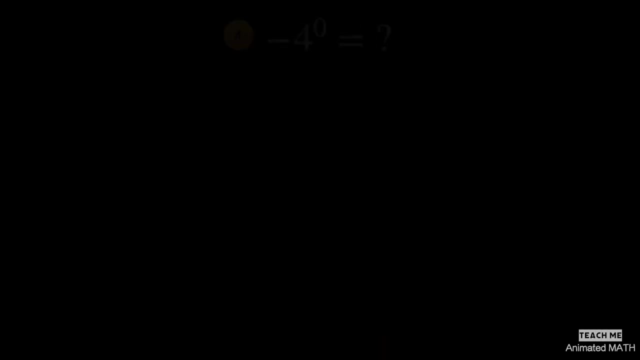 The base for the exponent of zero is 5x. By definition, the base 5x raised to the zeroth power is equal to 1.. This can be a little bit tricky. The base for the exponent of zero is 4,, not negative 4.. 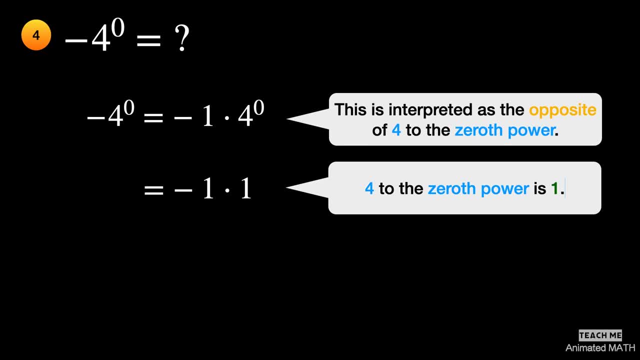 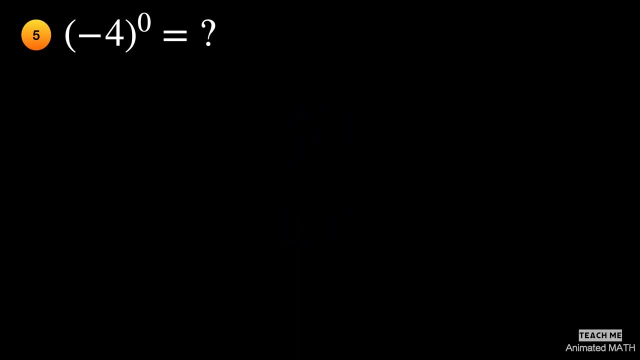 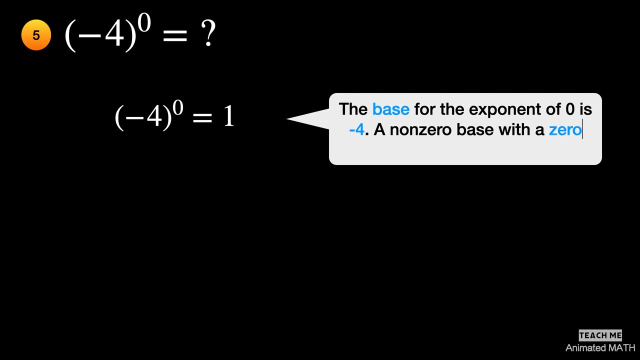 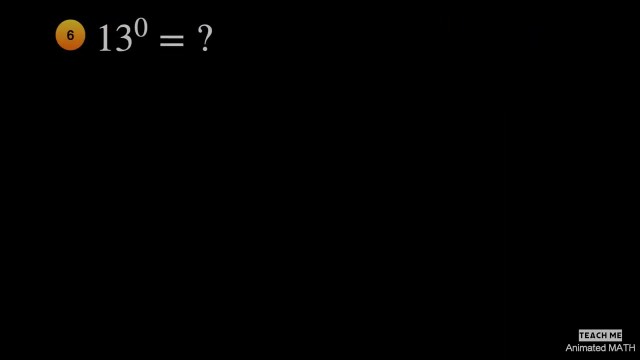 So 4 to the zeroth power is 1.. And the product of negative 1 and 1, is equal to negative 1.. The base for the exponent of zero is negative 4.. This means that the whole expression is equal to 1.. 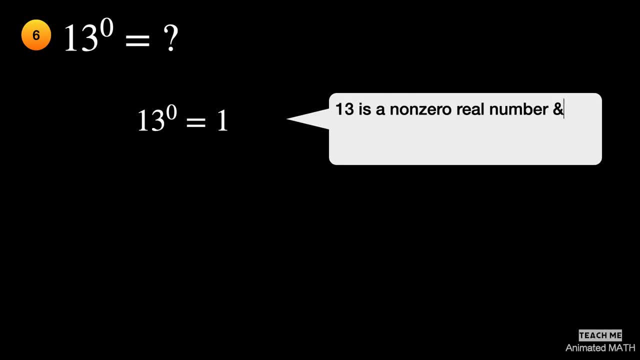 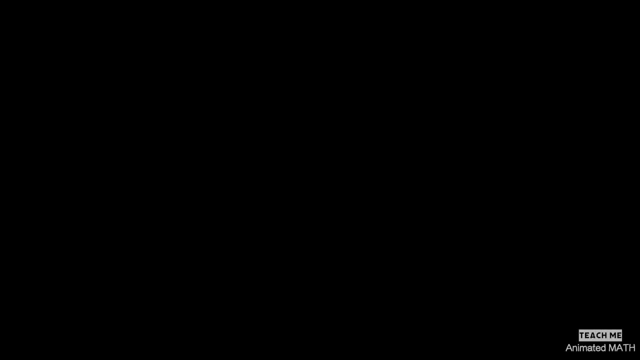 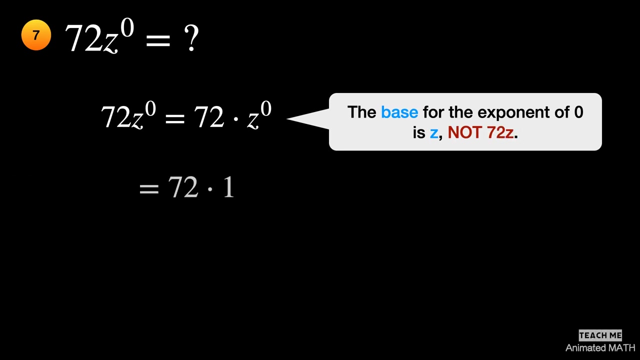 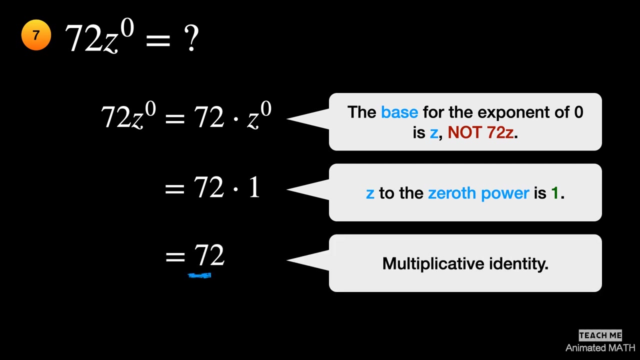 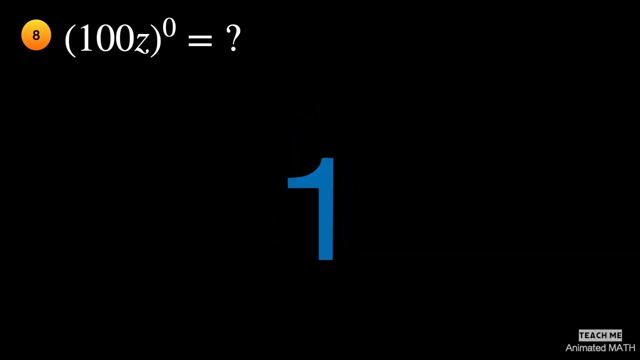 The base for the exponent of zero is 13.. So 13 to the zeroth power is equal to 1.. The base for the exponent of zero is z, not 72 z. The product of 72 and z raised to the zeroth power is 72 times 1, or 72.. 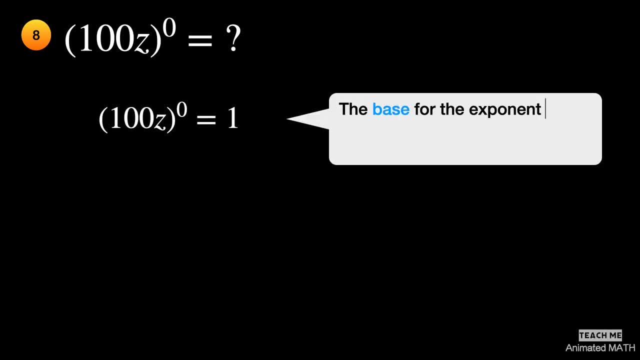 The base for the exponent of zero is 100 z By definition. the base 5x raised to the zeroth power is 1.. This can be a little bit tricky. The base for the exponent of zero is a third of the exponent of zero, so can belaim. 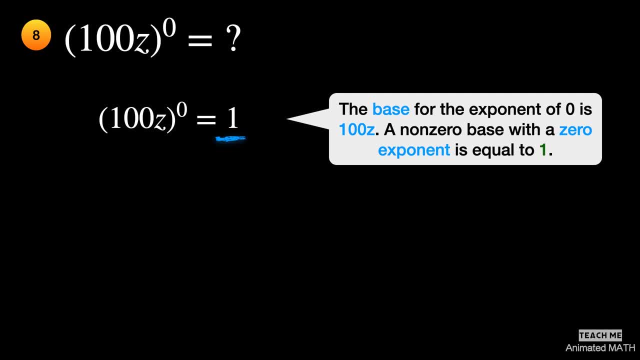 zero as 1.. The base for the exponent of zero is twice z. This can be very hard to understand, So the basic definition, the base 100 z raised to the zeroth power, is equal to 1.. 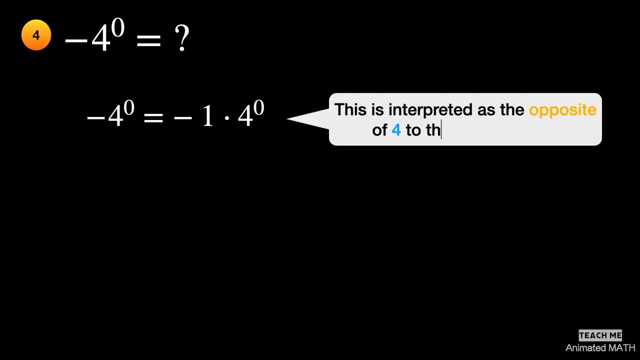 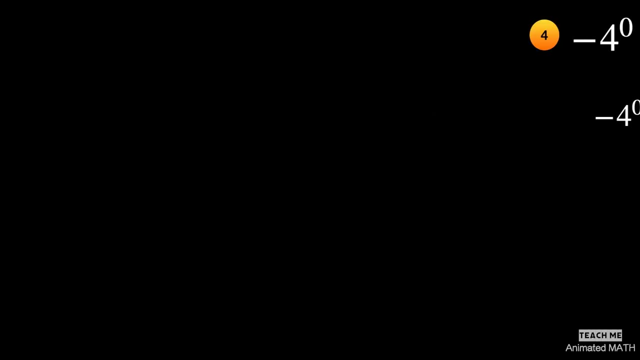 The base for the exponent of 0 is 4, not negative 4.. So 4 to the zeroth power is 1.. And the product of negative 1 and 1 is equal to negative 1.. The base for the exponent of 0 is negative 4.. 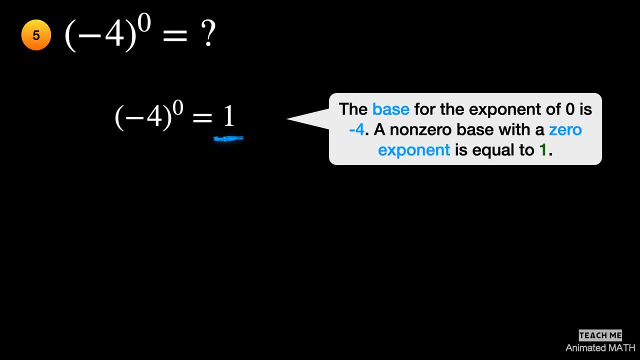 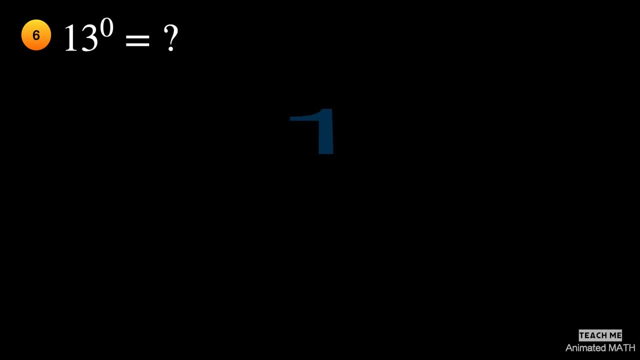 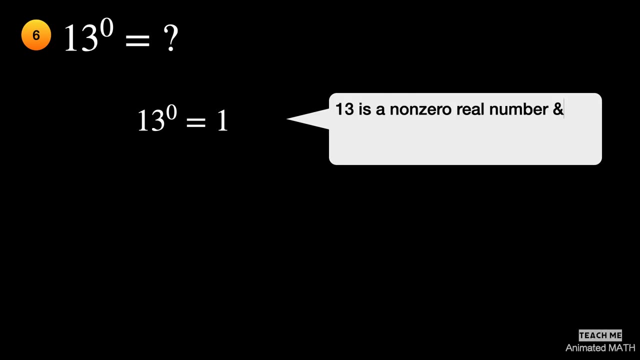 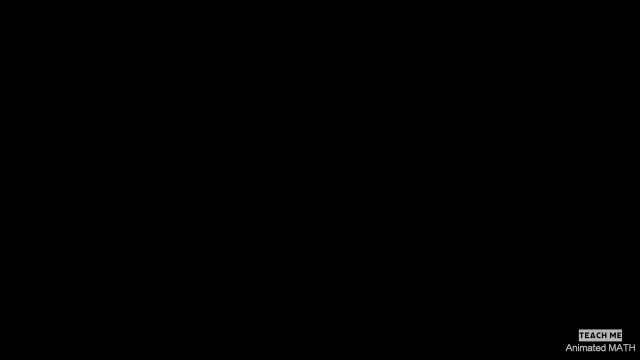 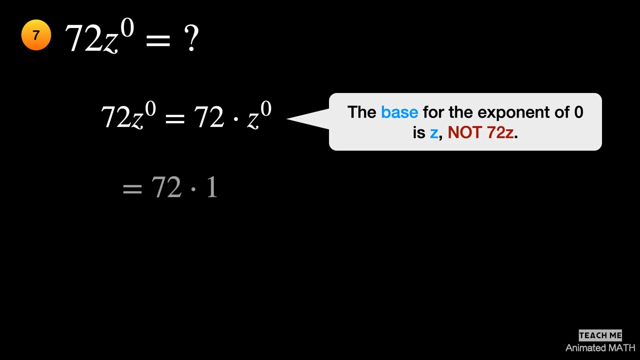 This means that the whole expression is equal to 1.. The base for the exponent of 0 is 13.. So 13 to the zeroth power is equal to 1.. The base for the exponent of 0 is z, not 72z. 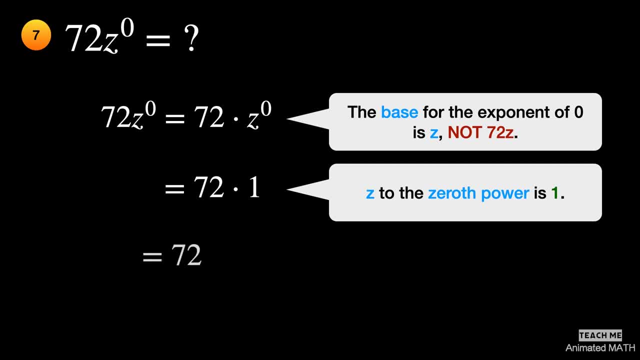 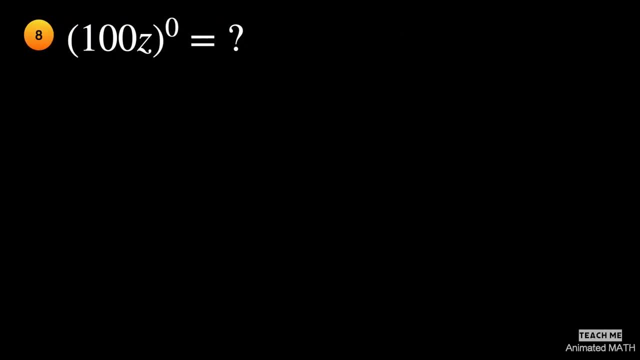 The product of 72 and z, raised to the zeroth power, is 72 times 1, or 72.. The base for the exponent of 0 is 100z. By definition, the base for the exponent of 0 is 100z. 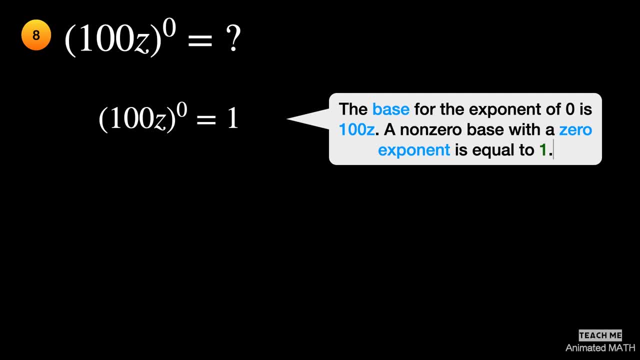 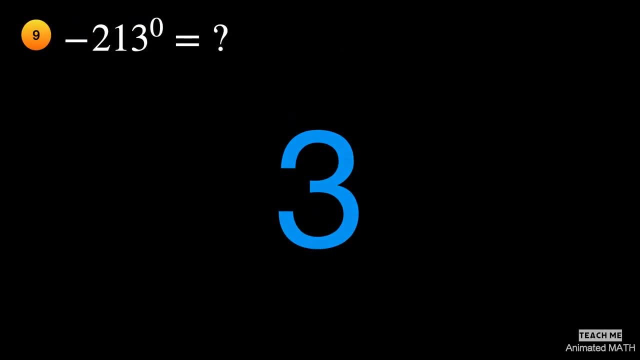 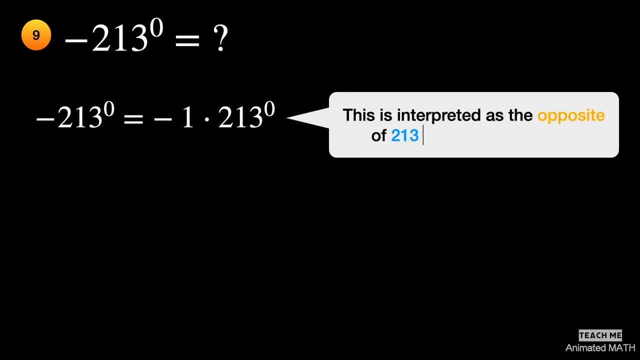 The base for the exponent of 0 is 100z. By definition, the base 100z raised to the zeroth power is equal to 1.. Don't be intimidated by this big number. Similar to an earlier problem, we solved. The base for the exponent of 0 is 213, not negative 213. 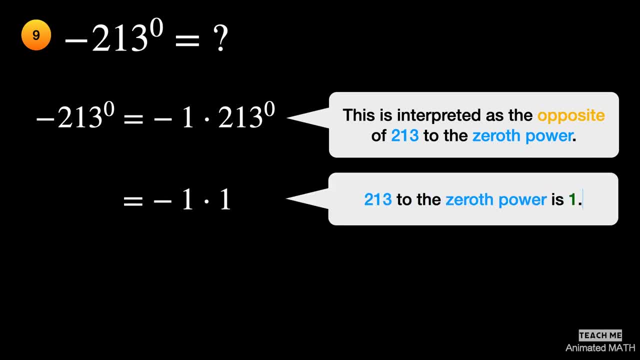 So 213 to the zeroth power is 1.. And the product of negative 1 and 1 is equal to negative 1.. Again, don't give in to the intimidation of big numbers. The base for the exponent of 0 is negative 365.. 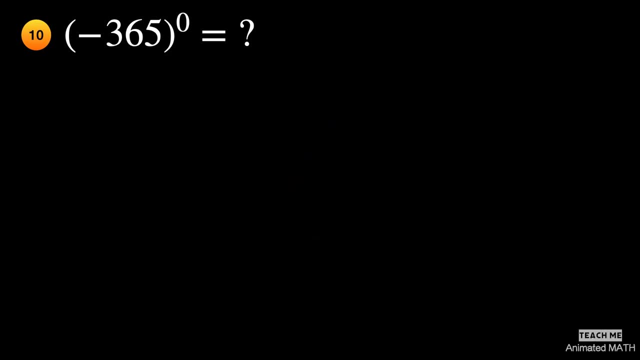 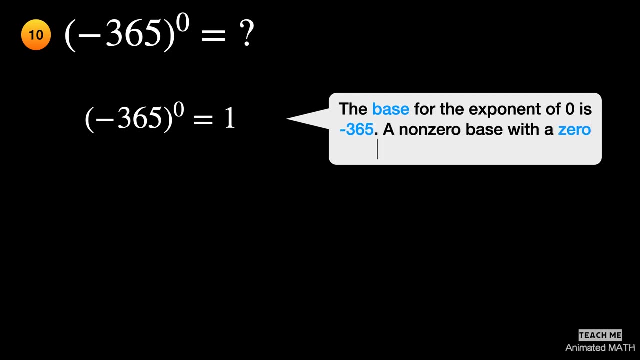 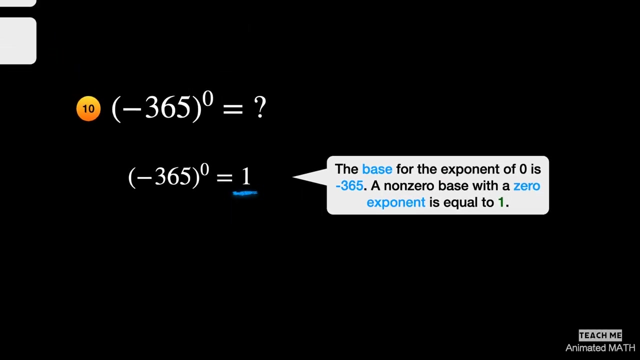 This means that the expression is equal to 1.. The base for the exponent of 0 is negative 325,. this means that the expression is equal to 1.. And there you have it. I hope you learned a lot in this solve-along video about zero exponents.